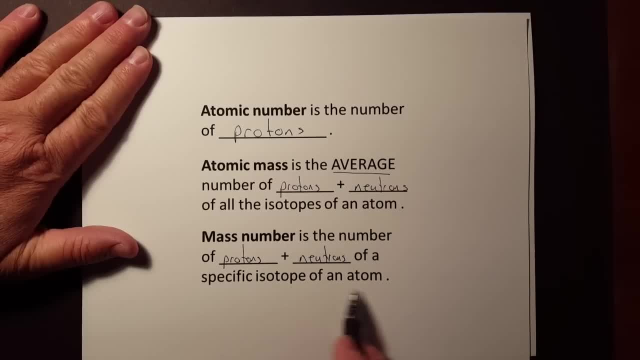 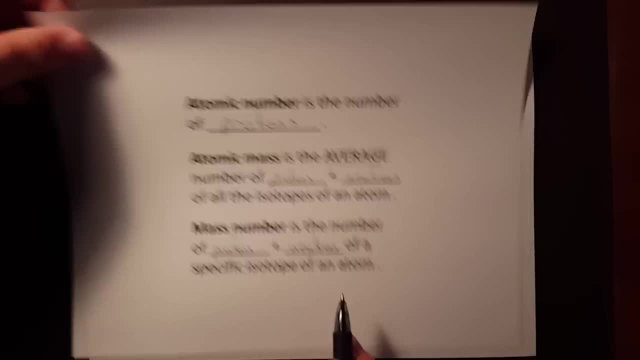 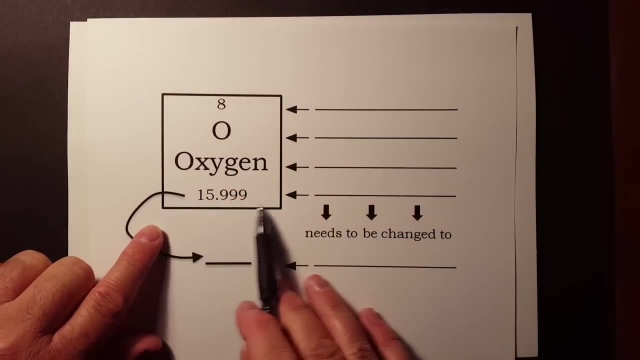 but this time only of one particular isotope of the atom, Any one all-by-itself atom. its mass number is protons plus neutrons. Now, what does that show us then? Let's take a look. This is a box that we would find in the periodic table for oxygen. 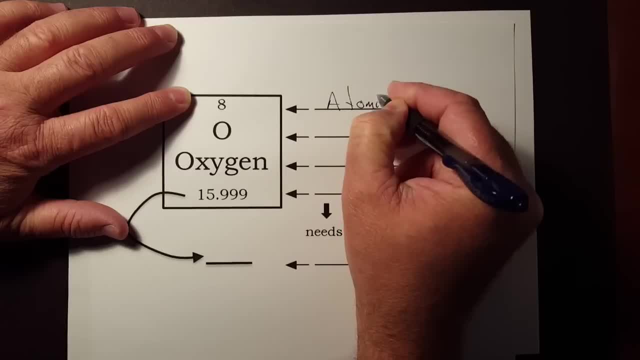 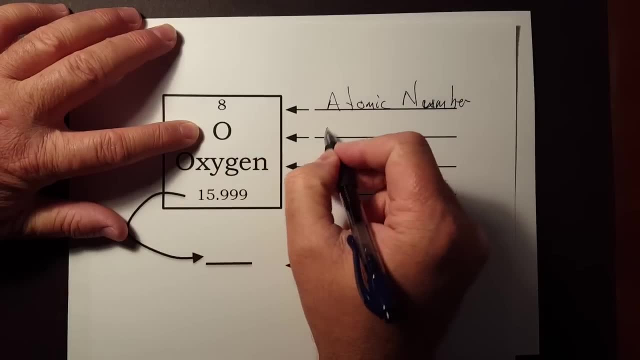 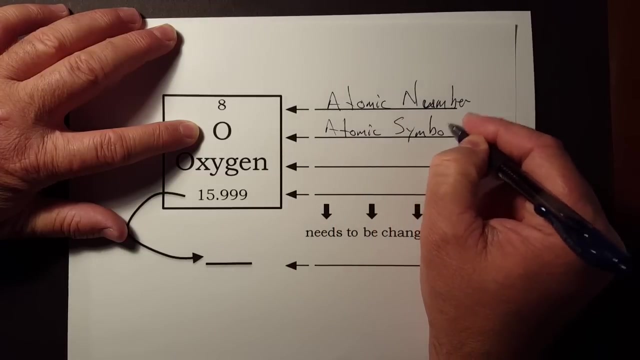 The number at the top is always the atomic number. That's how many protons we have Down here we have the atomic symbol. Now, in this case, remember, uppercase and lowercase makes a very big difference. Below it we're going to have the name. 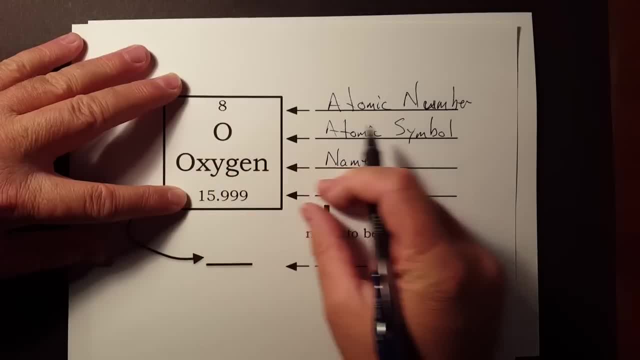 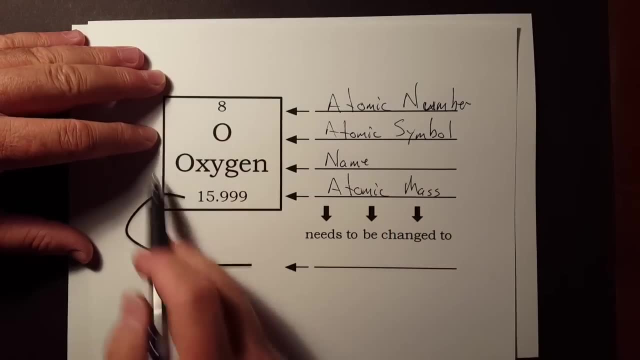 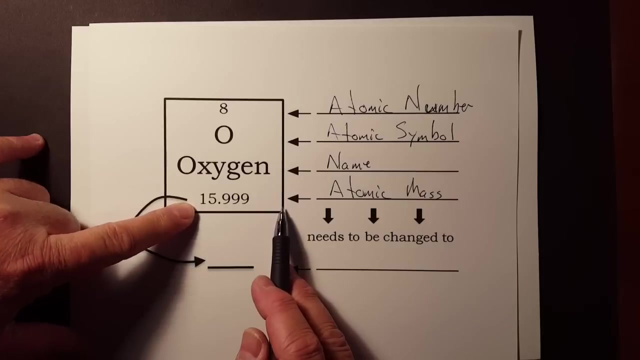 and at the bottom, because there's all the decimals, this is the atomic mass. That's what we're given, but what we can find from this is a lot more information. So, for instance, if we take the mass and we round it to the nearest whole number, 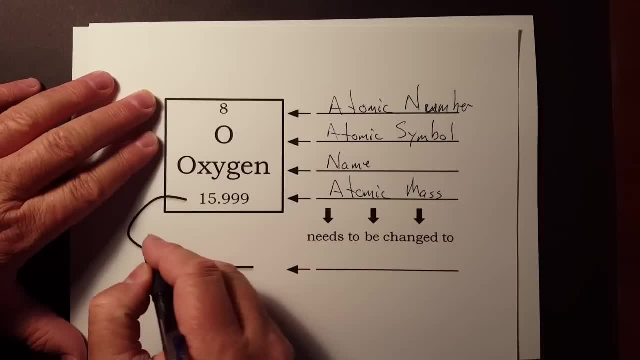 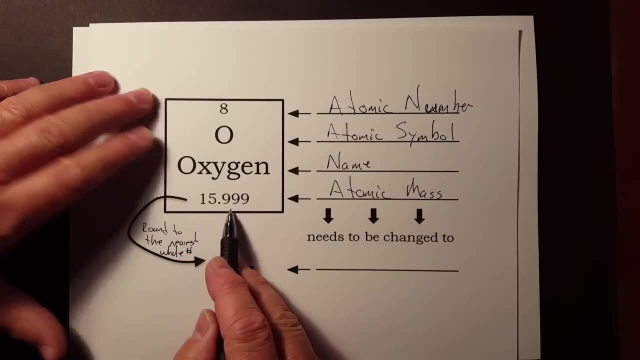 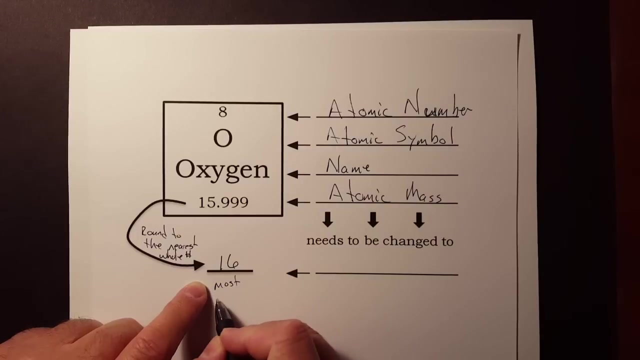 Now 15.9,. we don't really care about the extra nines. so if we're going to round to the nearest whole number, that would be 16.. Because this is all the different isotopes taken in for for the average. the nearest whole number is the most common variety. 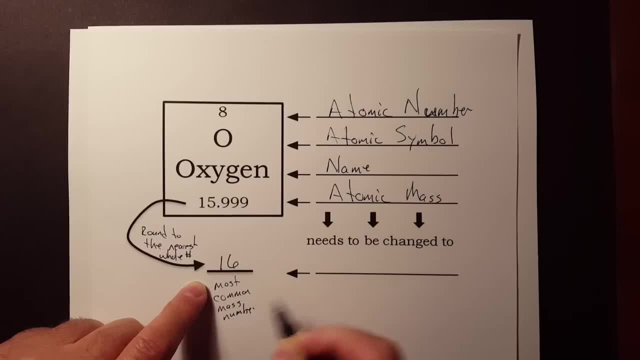 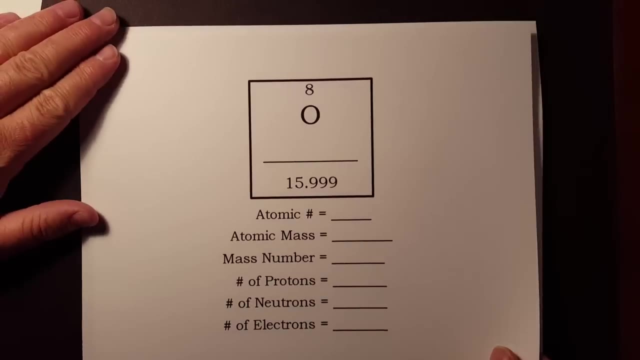 So that's going to be the most common mass number, That's protons plus neutrons. So let's take a look from our worksheet, The first one. we're dealing with oxygen. again We see in the box the one thing that's missing. 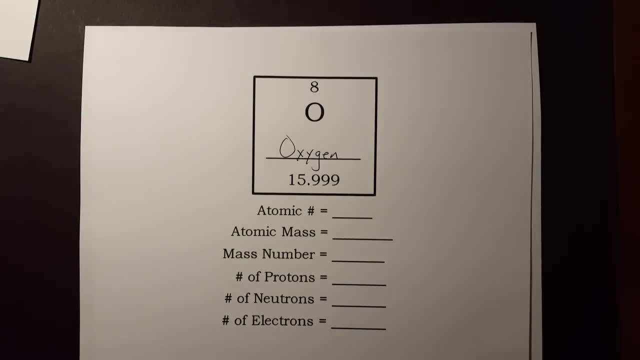 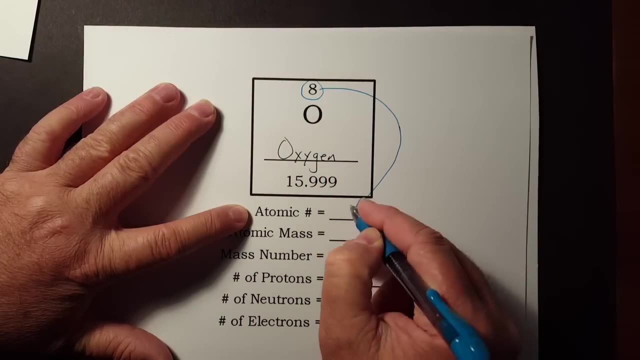 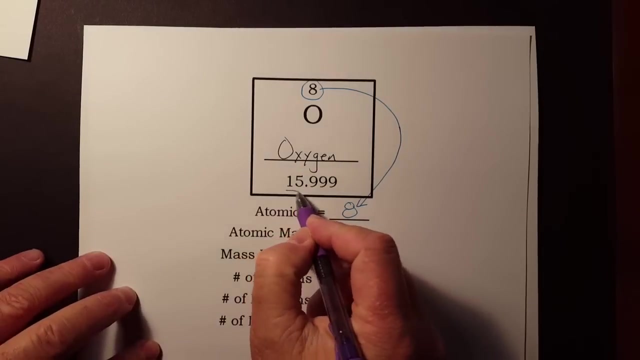 It's the name. Now, from here, let's take a look. The atomic number we're always going to find up top, So we're just going to bring that down. The atomic mass is the one that has all of the decimals. 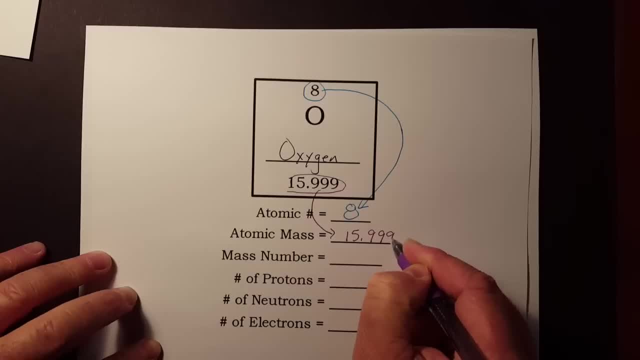 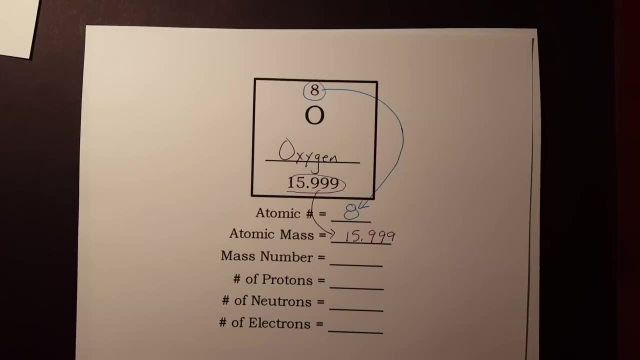 We'll bring it down also 15.999.. Now the mass number. we want that to be rounded from the nearest whole number, So 15.9,. again, we don't care about the extra nines. that rounds to 16.. 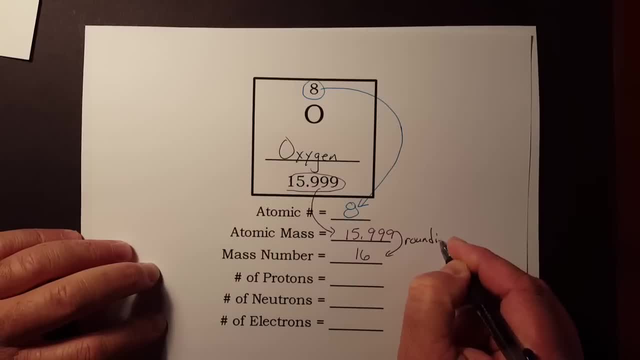 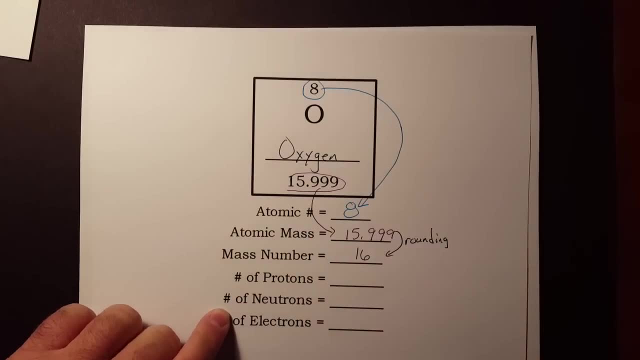 We found that by rounding Now from here, we're going to be able to figure out the protons, neutrons and electrons. given these numbers, The first one is pretty simple: The atomic number, by its definition, is the number of protons. 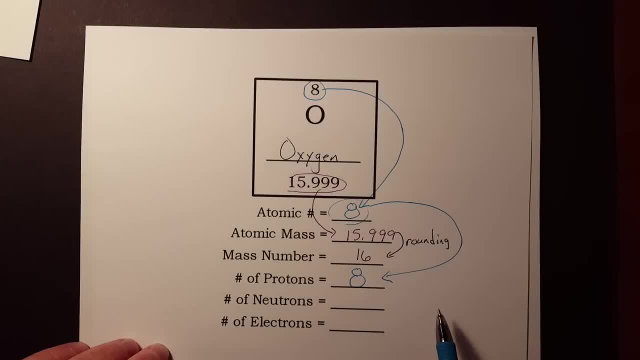 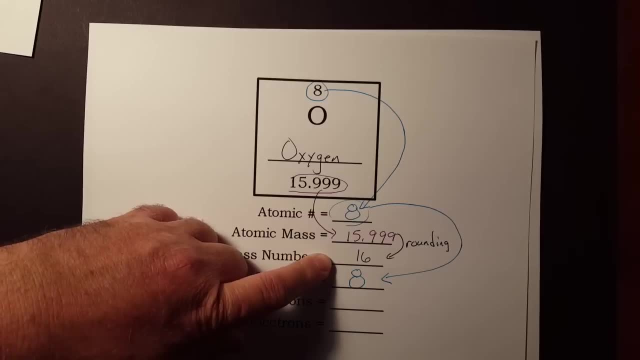 And the mass number, Since that is protons plus neutrons. what we need to do is say: here's a complicated math: if 16, that was our protons plus the number of neutrons, we already know that protons was 8.. 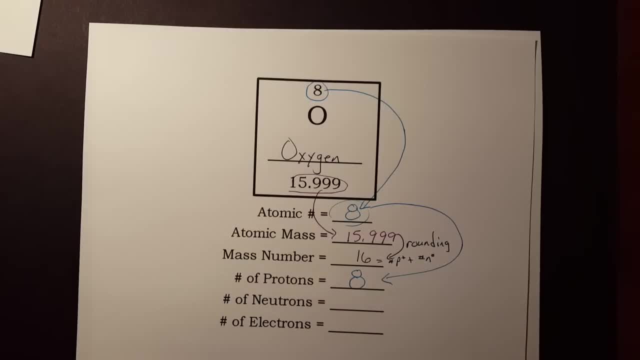 So 16 is 8, plus what number? Well, in this case, pretty simple, that's another 8.. The periodic table of elements is always going to represent the atom in its neutral state, meaning it doesn't have a plus or a minus charge. 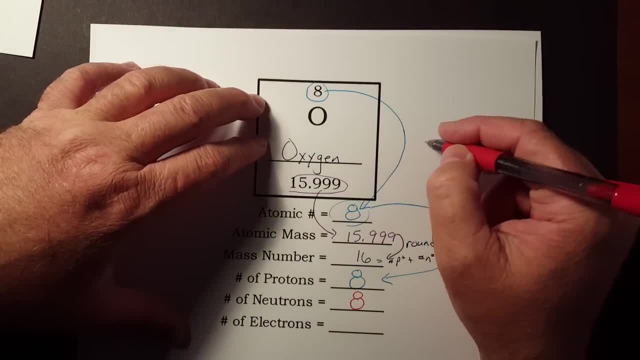 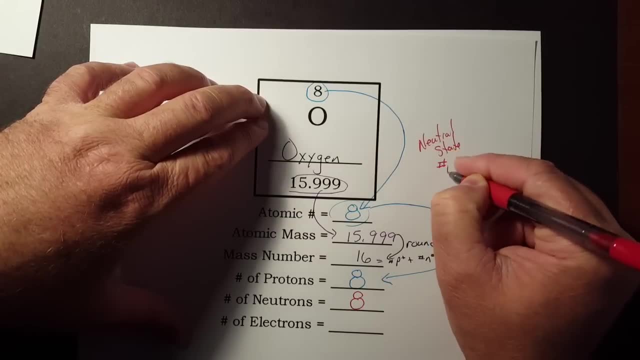 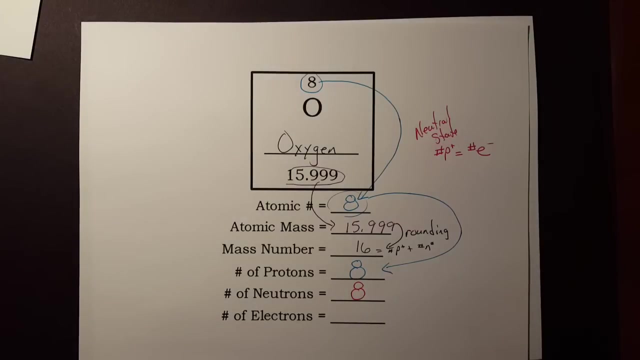 Remember, the pluses come from the protons. So in its neutral state, the number of protons always equals the number of electrons. So if we have 8 protons, I'm going to use blue again because again, I'm just going to bring it down. 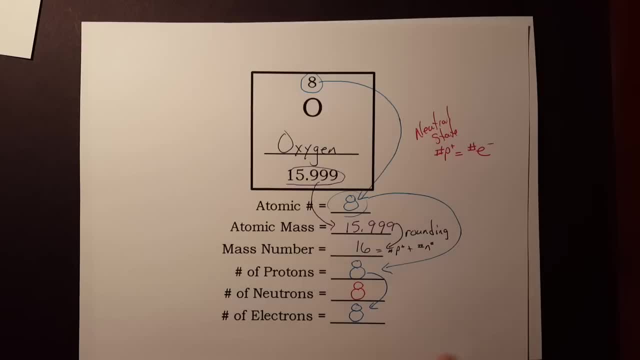 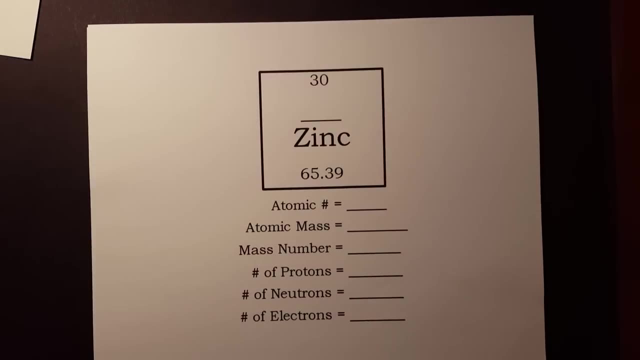 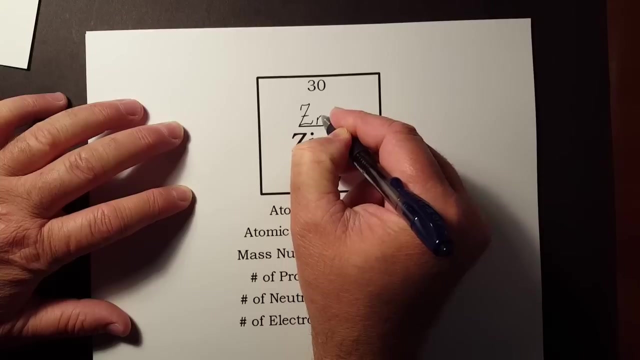 That means oxygen has to also have 8 electrons. All right, let's take a look at our next example, Our next example, number 30 on the periodic table. What we're missing is zinc capital Z lowercase, n, Notice lowercase, not just a capital N made smaller. 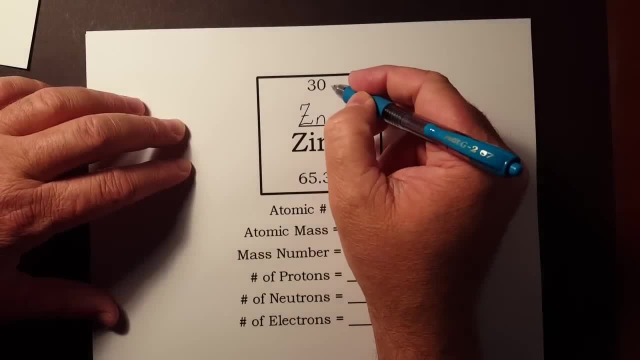 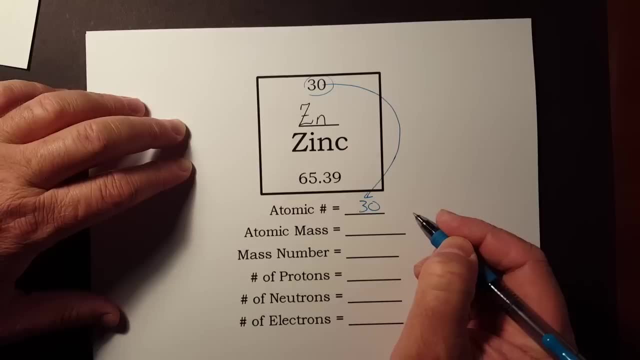 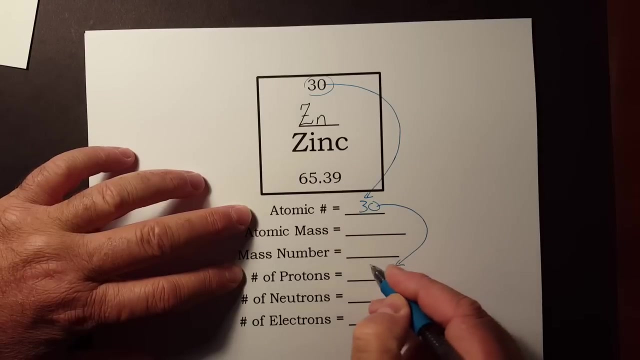 It makes a difference. We're going to start again. We take our atomic number. that is straight from the top. We're going to slip around here and make our life a little bit easier, Since we already know the atomic number. we already know that that's the number of protons. 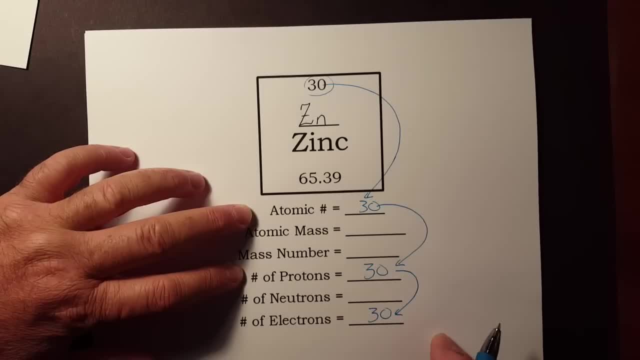 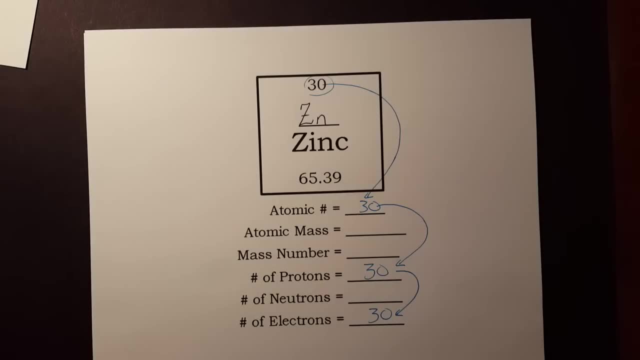 And since it's a neutral atom, we already know that has to be the same as the number of electrons. So right away, that number gives us three things. to fill in The atomic mass We need all the decimals: 65.39..